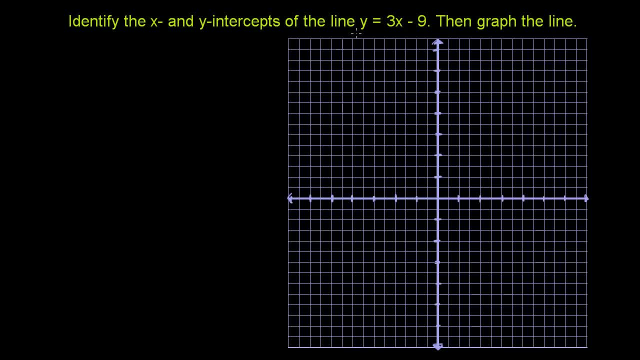 Identify the x and y intercepts of the line. y is equal to 3x minus 9.. Then graph the line, So the x-intercept. I'll just abbreviate it as x? int. that is where the line intersects the x-axis. 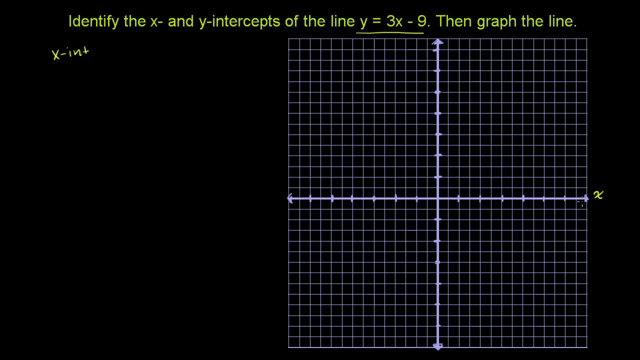 So where it intersects the x-axis- Remember this horizontal axis- is the x-axis. So when something intersects the x-axis, what do we know about its coordinate? Its x value could be anything, but we know its y value is 0.. 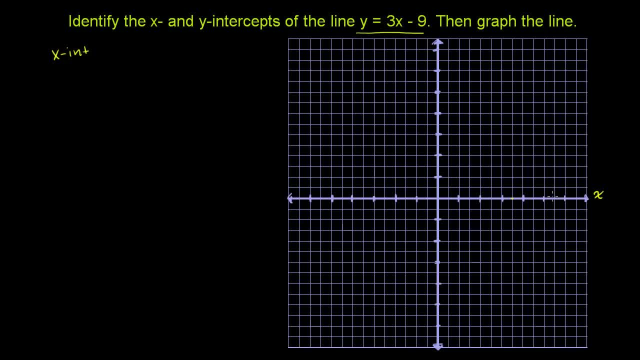 If we're intersecting, if we're sitting on the x-axis someplace, that means that we haven't moved in the y direction. That means that y is 0. So this means literally that y is 0. So we need to find the x value defined by this relationship. 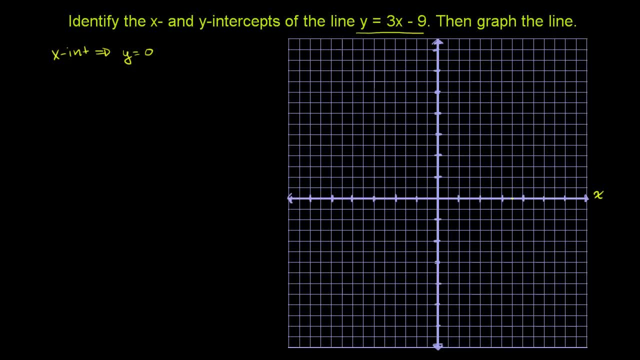 when y is equal to 0.. Similarly, when we talk about the y-intercept- I'll do it down here: When we talk about the y-intercept, what does that mean? Well, y-intercept means so this is the y-axis right over here. 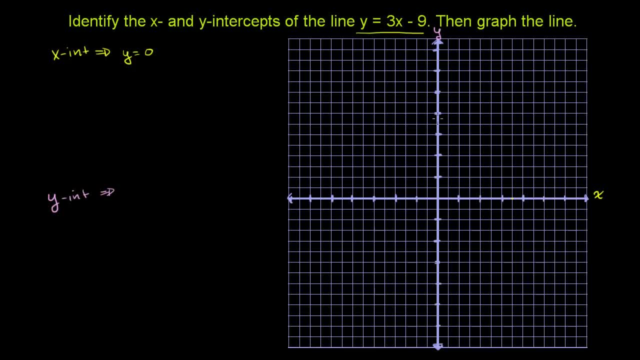 running up and down. The y-intercept is the point at which the line intercepts the y-axis. So what's going on? If we're at the y-axis, our y value could be anything depending on where we intersect the y-axis. 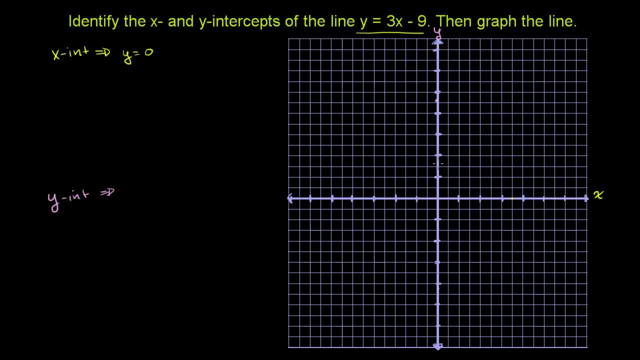 But we know that we haven't moved to the right or the left. We know that our x value is 0 at the y-intercept, So over here our x value is going to be 0. And to find the actual point, we just 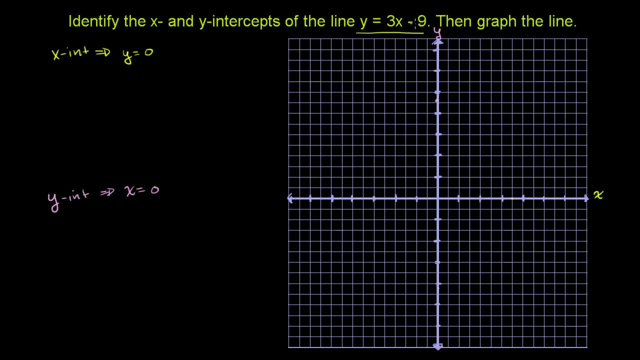 have to find the corresponding y value defined by this relationship or this equation. So let's do the first one. first, The x-intercept is when y is equal to 0.. So we set y is equal to 0, and then we'll solve for x. 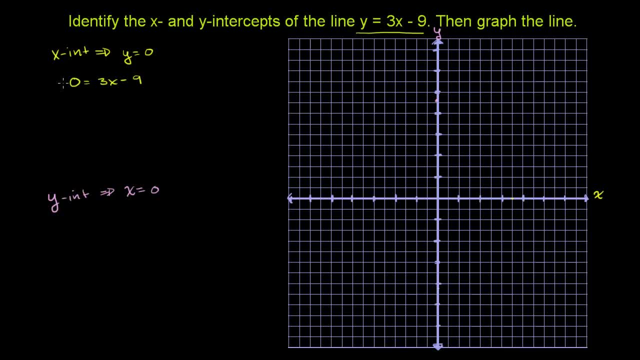 So we get 0 is equal to 3x minus 9.. We can add 9 to both sides of this equation to isolate the x term. So we get 9 is equal to 3x. These cancel out. We could divide both sides by 3.. 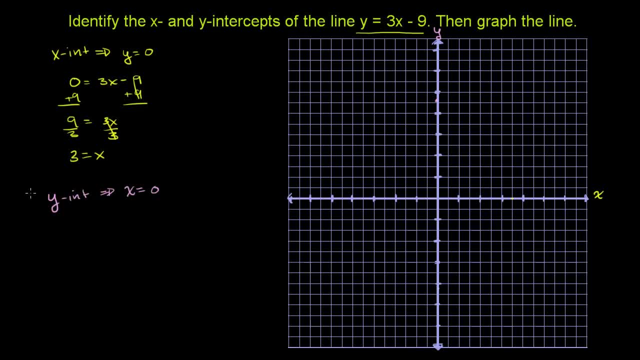 We get: 3 is equal to x or x is equal to 3.. So the point y is equal to 0,, x is equal to 3 is on this line And let me put it in order: The x-coordinate always goes first. 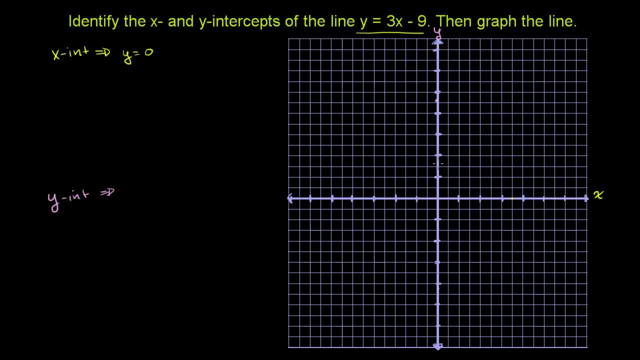 But we know that we haven't moved to the right or the left. We know that our x value is 0 at the y-intercept, So over here our x value is going to be 0. And to find the actual point, we just 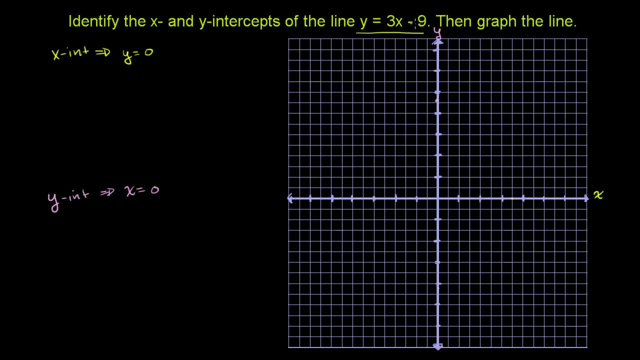 have to find the corresponding y value defined by this relationship or this equation. So let's do the first one. first, The x-intercept is when y is equal to 0.. So we set y is equal to 0, and then we'll solve for x. 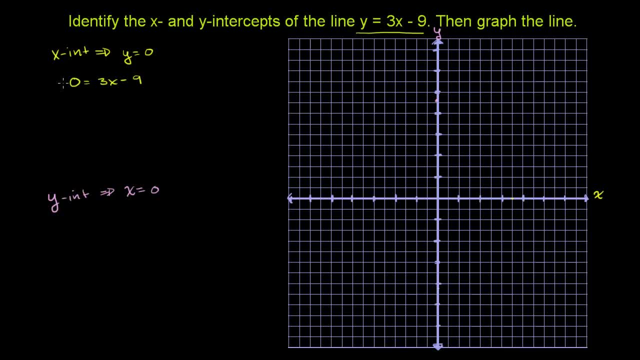 So we get 0 is equal to 3x minus 9.. We can add 9 to both sides of this equation to isolate the x term. So we get 9 is equal to 3x. These cancel out. We could divide both sides by 3.. 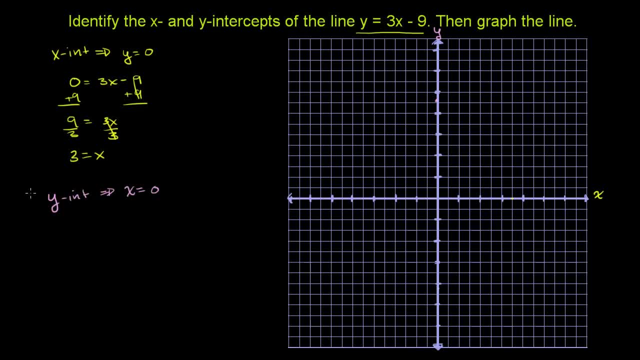 We get: 3 is equal to x or x is equal to 3.. So the point y is equal to 0,, x is equal to 3 is on this line And let me put it in order: The x-coordinate always goes first. 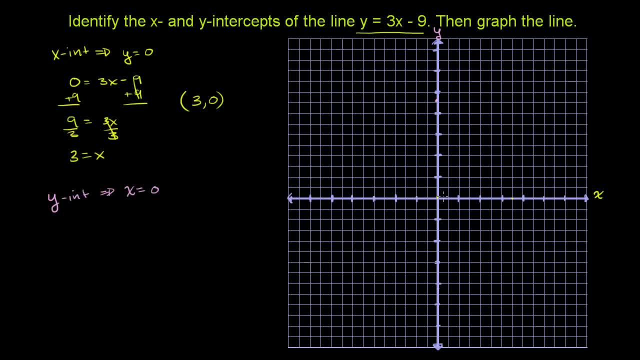 So it's 3 comma 0.. So this is the origin: 1,, 2,, 3 is right over here. That is 3 comma 0.. This right here is the x-intercept And remember, notice- that point lies on the x-axis. 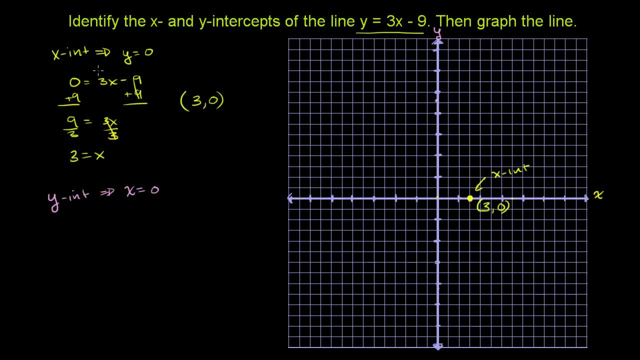 But the y value is 0. We haven't moved up or down. When you think x-intercept, you say, OK, that means my y value is 0. So I have to solve for the x value. Now we do the opposite for the y-intercept. 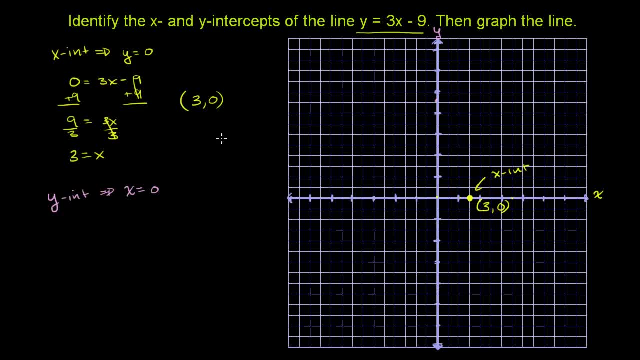 And the y-intercept. We're sitting on this line. x value must be 0. So let's figure out what y is equal to when x is equal to 0. So y is equal to. I want to do it in that pink color. 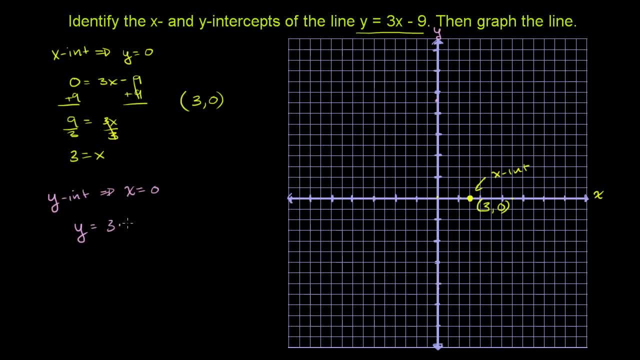 y is equal to 3 times x is 0. now, 3 times 0 minus 9.. Well, 3 times 0 is just 0. So 0 minus 9, well, that's just equal to negative 9.. 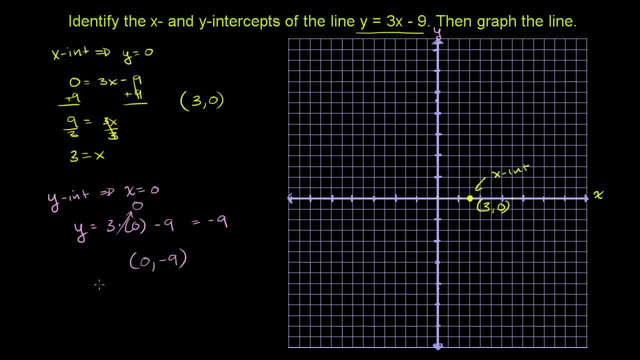 So we have the point 0, comma, negative 9.. So when x is 0, we go down 9 for y: 1,, 2,, 3,, 4,, 5,, 6,, 7,, 8,, 9.. 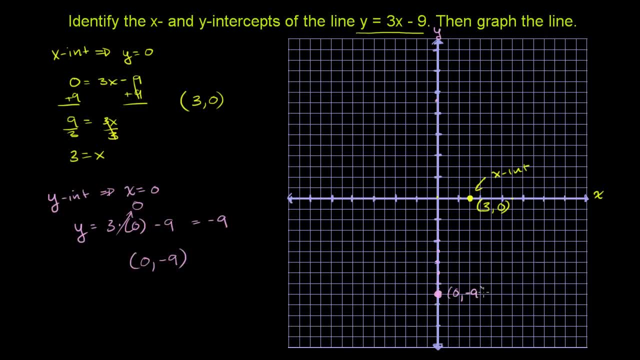 So right, there is the point 0, comma, negative 9.. Notice, it sits on the y-axis, That's why it's the y-intercept And the x value is 0.. We haven't moved to the left or the right. 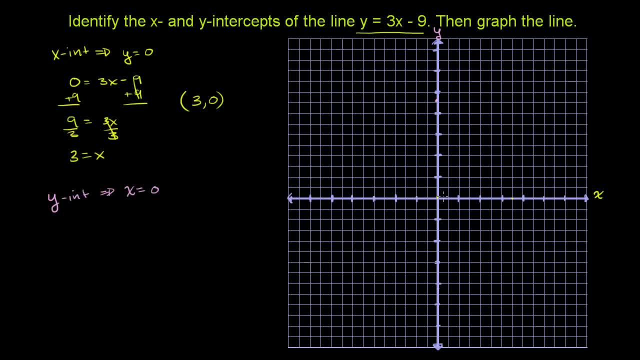 So it's 3 comma 0.. So this is the origin: 1,, 2,, 3 is right over here. That is 3 comma 0.. This right here is the x-intercept And remember, notice- that point lies on the x-axis. 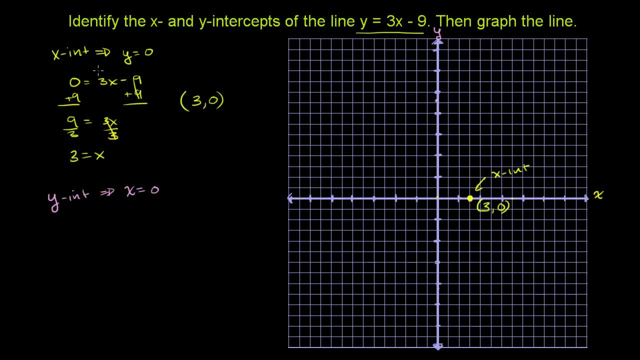 But the y value is 0. We haven't moved up or down. When you think x-intercept, you say, OK, that means my y value is 0. So I have to solve for the x value. Now we do the opposite for the y-intercept. 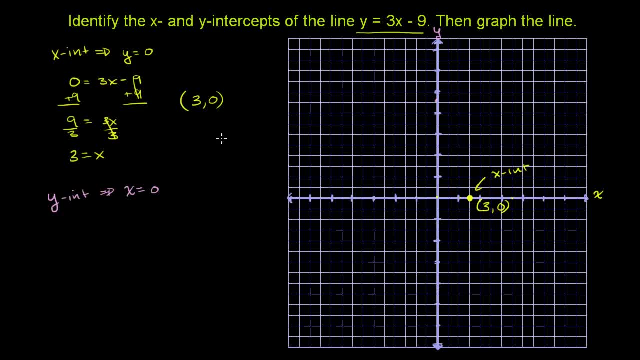 And the y-intercept. We're sitting on this line. x value must be 0. So let's figure out what y is equal to when x is equal to 0. So y is equal to. I want to do it in that pink color. 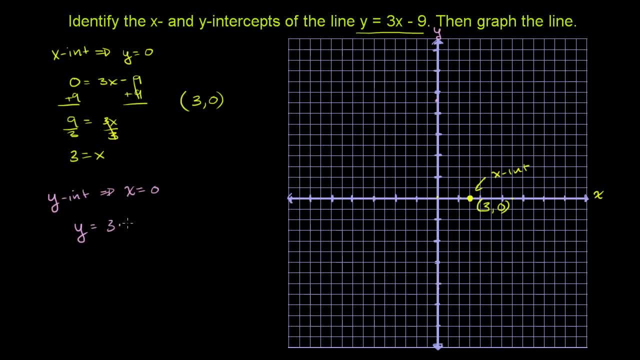 y is equal to 3 times x is 0. now, 3 times 0 minus 9.. Well, 3 times 0 is just 0. So 0 minus 9, well, that's just equal to negative 9.. 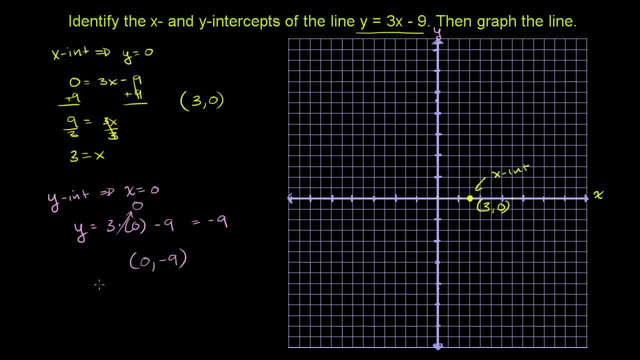 So we have the point 0, comma, negative 9.. So when x is 0, we go down 9 for y: 1,, 2,, 3,, 4,, 5,, 6,, 7,, 8,, 9.. 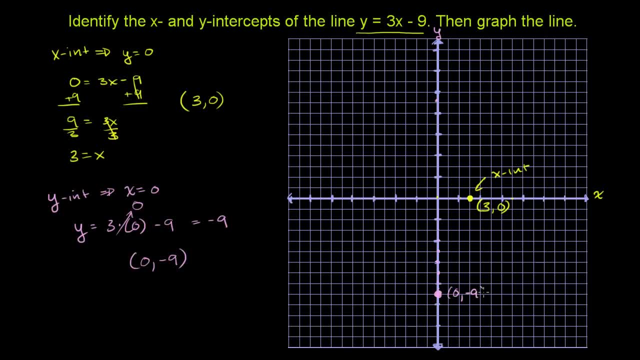 So right, there is the point 0, comma, negative 9.. Notice, it sits on the y-axis, That's why it's the y-intercept And the x value is 0.. We haven't moved to the left or the right. 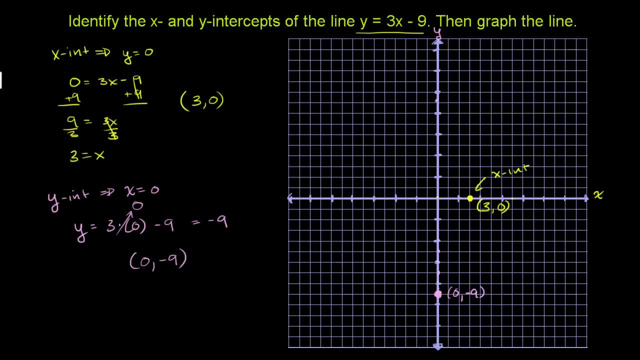 All you need is two points for a line. So we're now ready to graph. We essentially just have to connect the dots. So it's going to look something like this. It's going to look something our line. I don't have a good line tool, so I'm going to draw you. 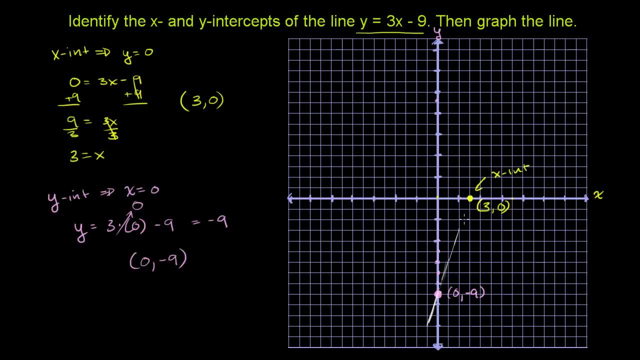 my best to draw it nicely. It is going to look something like that: And you just keep going, You just keep going. You want to do a straight line, So it just keeps going on and on and on like that. And I could keep going all the way in that direction. 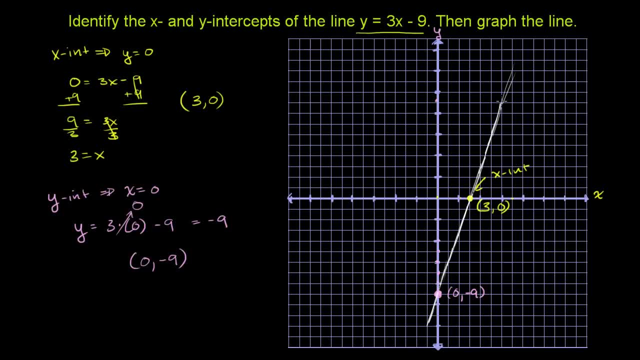 But then my line doesn't look as straight all of a sudden. I think you get the general idea. I could keep going like that and then keep going like that. I don't have a nice ruler to do it with, And we're done. All right.